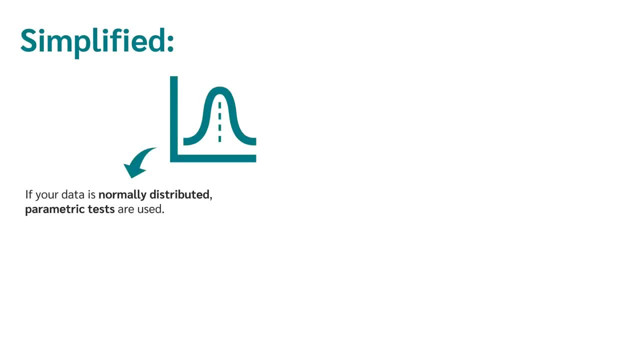 if your data are normally distributed, you use a parametric test In the case of two dependent samples. this is the t-test for dependent samples. If your data is not normally distributed, you use a non-parametric test In the case of two dependent samples. this would be the Wilcoxon. 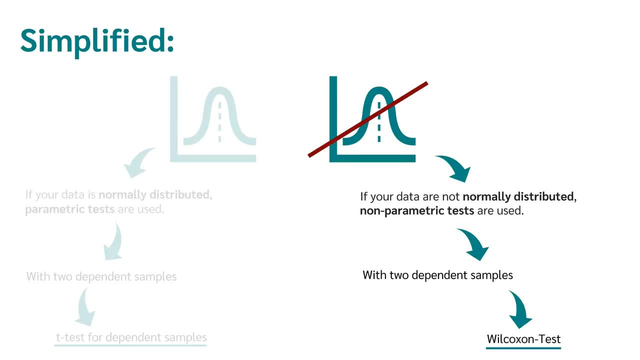 test. Now, of course, you could say: well then I'll just always use the Wilcoxon test and I don't even have to check the normal distribution. At the end of this video I will show you why you should always use the t-test, if it's possible to do so. 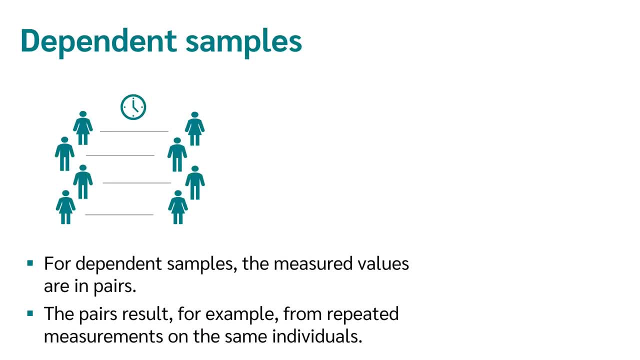 First I have a little reminder for you what dependent samples are. In dependent samples the measured values are always available in pairs. The pairs result from, for example, repeated measures of the same person. But what is the difference now between the t-test for? 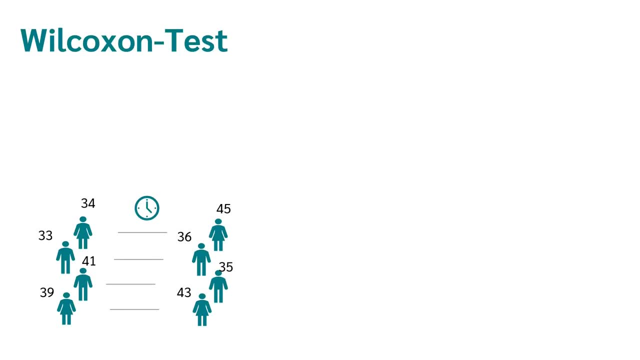 dependent samples and the Wilcoxon test- The t-test for dependent samples- tests whether there's a difference in means. If we have a dependent sample- say we took a value from each person once in the morning and once in the evening- then we can calculate the difference from each pair. So, for example, 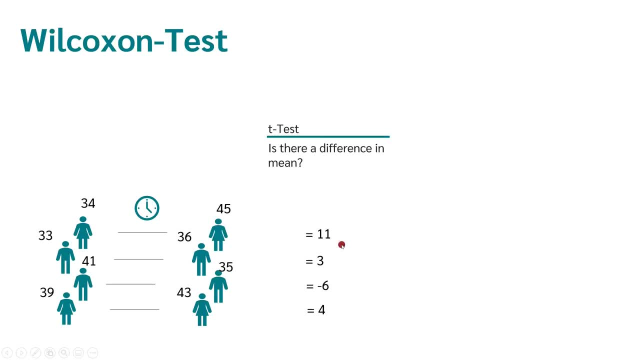 we would have 45 minus 34,, which equals 11.. The t-test for dependent sample now tests whether these differences differ from zero or not. In the Wilcoxon test we don't use the differences of means, but we form ranks and then we compare these ranks with. 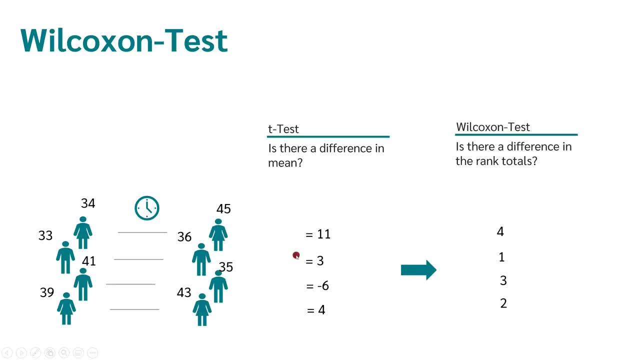 each other. Three is the smallest value in terms of amount. It gets rank one. Four is the second smallest value and it gets rank two. Six gets rank three and 11 gets rank four. We assign a plus to all positive values and we get a plus to all positive values, So we have a plus to all. 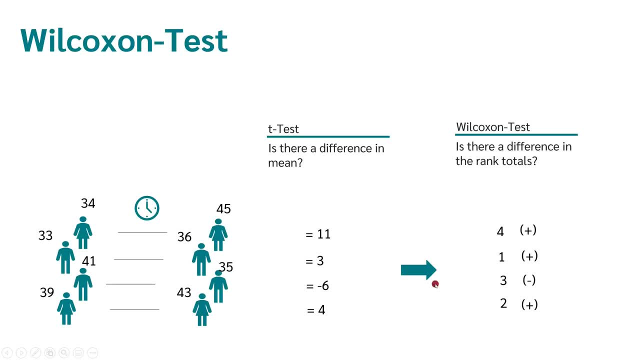 positive values and we get a plus to all positive values. So we have a plus to all positive values. So we have a plus to all positive values and a minus to all negative values. But don't worry, we will go through this slowly and we'll also look at an example. 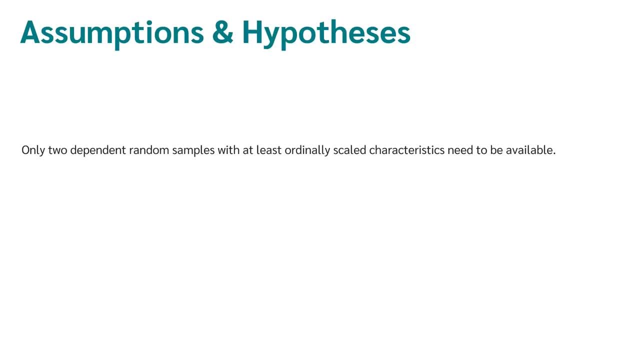 Now we go to the assumptions and the hypotheses. In the Wilcoxon test, only two dependent random samples with at least ordinarily scaled characteristics need to be present. The variables do not have to satisfy a distribution curve. What should be mentioned now, however, is that the distribution shape of the differences of the two dependent samples 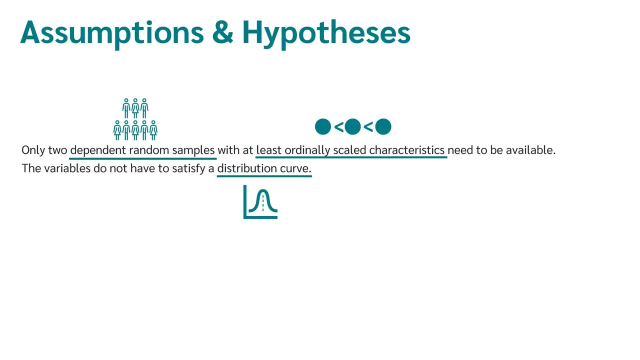 should be approximately symmetric. The null hypothesis in a Wilcoxon test is that there is no difference in the so-called central tendency of the two samples in the population. That is, that there's no difference between the dependent groups. The alternative hypothesis is that there is no difference between the dependent groups. The alternative hypothesis is that there is no one знач. 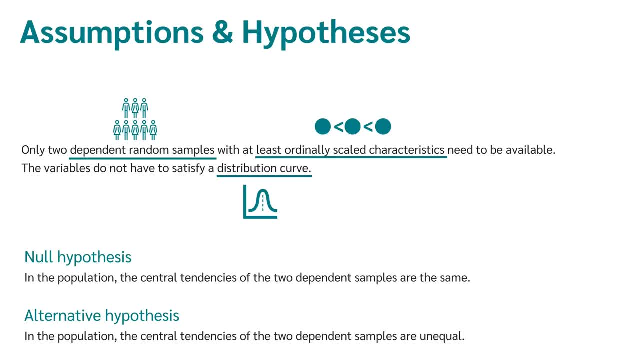 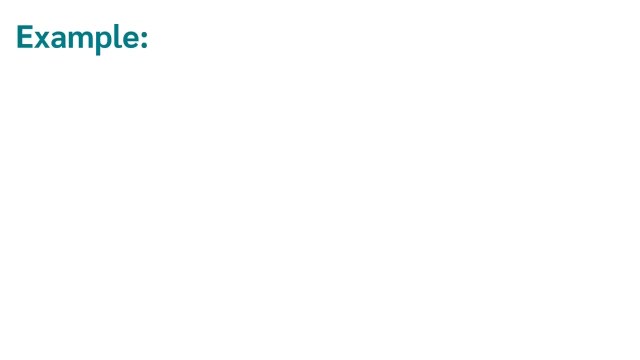 The autonomous group Wen is a difference in the central tendency in the population, so we expect that the two dependent groups are different. So now we finally look at a quite simple example. Let's say you have measured the reaction time of a small group of people once in the morning and once in the evening. 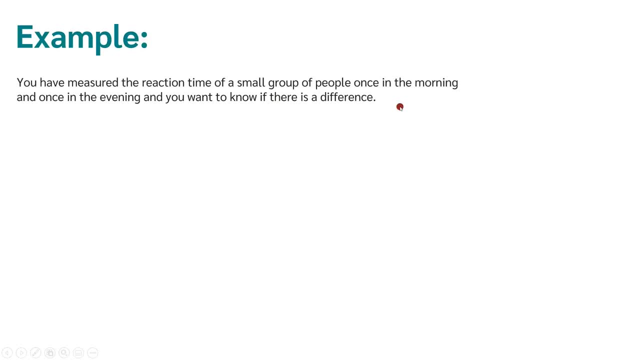 and you want to know if there is a difference between morning and evening. In order to do this, you measure the reaction time of seven people in the morning and in the evening. The measured values are therefore available now in pairs, And now you want to calculate the difference between morning. 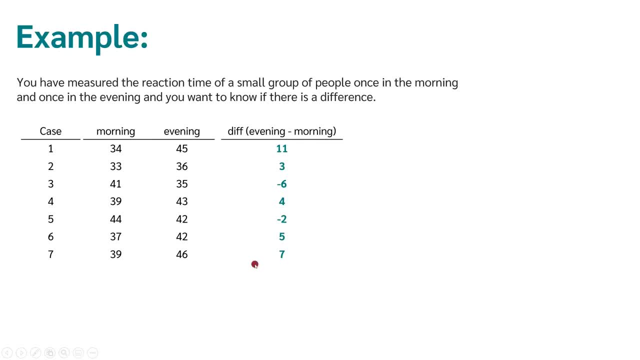 and evening. If the difference would be normally distributed, you would use a t-test for dependent samples. If it is not, we would use a Wilcoxon test. Let's just assume that there is no normal distribution. If it is not, we would use a Wilcoxon test. Let's just assume that there is no normal distribution. 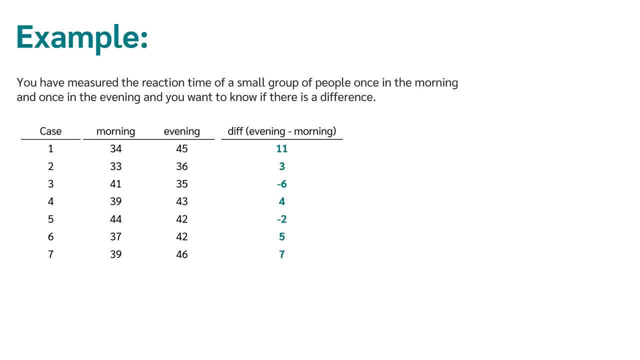 And we need to calculate a Wilcoxon test In order to do this. the first thing we do is we form ranks. We look for the smallest value in terms of amount, that is minus 2, which gets rank 1.. What is the second smallest value? That is 3, which gets rank 2, and so on and so forth until we have. 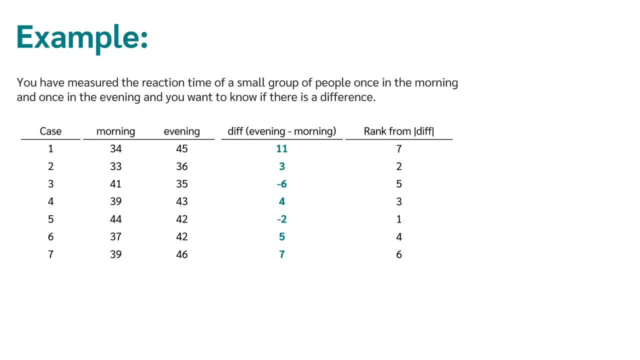 ranked all the values. The next thing is that we have to calculate the number of people in the group. So the first thing is that we look at the differences and we try to figure out which difference is positive and which is a negative one. For the negative differences, we simply 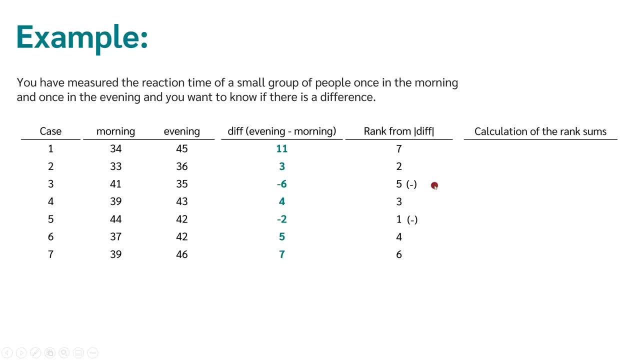 add a minus, Then we can add up the positive ranks and the negative ranks. For the positive ranks, we get 7 plus 2 plus 3, plus 4, plus 6, which is equal to 22.. For the negative ranks, we get 15.. For the positive: ranks, we get 5 plus 1, which is equal to 6.. If there is no difference between morning and evening, the positive and negative ranks should be approximately equal. Therefore, the null hypothesis is that both rank sums are equal. But how can we test this? Now we have the sum of ranks. 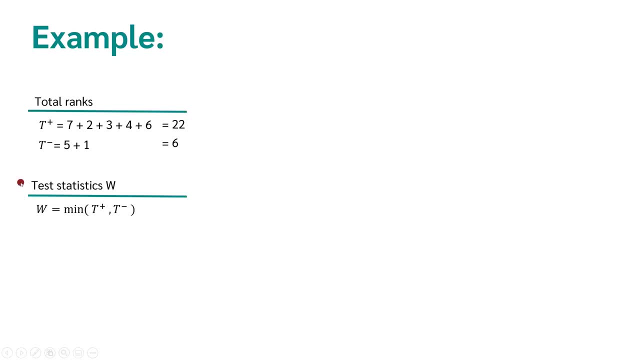 and we use it to calculate the test statistic w. This is simply the minimum value of t plus and t minus. In our case, it is the minimum value of 22 and 6 and therefore the test statistic w in our case is 6.. Now we can further calculate the value for t or w that we would expect if there was no difference between morning and evening. Now we can further calculate the value for t or w that we would expect if there was no difference between morning and evening. Now we can further calculate the value for t or w that we would expect if there was no difference between morning and evening. 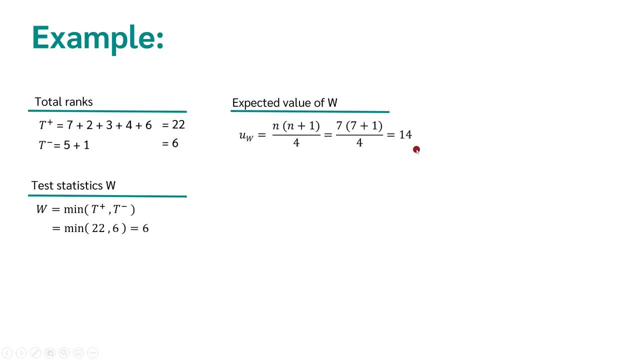 In this case, we would get a value of 14.. In this case, we would get a value of 14.. Therefore, if there is no difference between morning and evening, we would actually expect a value for t plus and t minus of 14, and thus w would also be 14.. Further we can calculate. 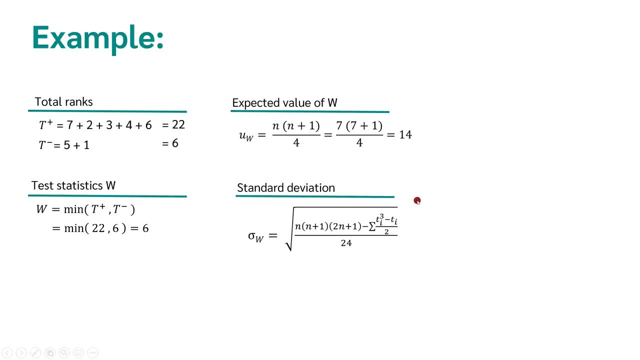 the standard deviation. This is given by this, to be fair, a little bit complicated formula. Once we have found the expansion, shallainen states the value for t or w. These variables that we data our perform parcels either as 1.1 or 0.2, and ie 0.0 as a function. 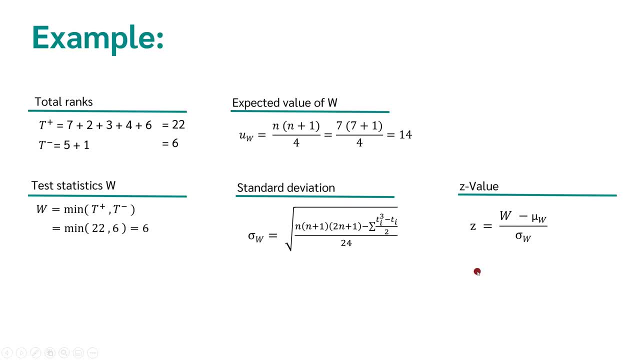 So let us consider w as 4.. Since the integral is, in teens, less than 1.8 and 1.4 for ma English, We also need to separate this by creating a new variable for q. finished with that, we can now calculate the Z-value. The Z-value is obtained by calculating. 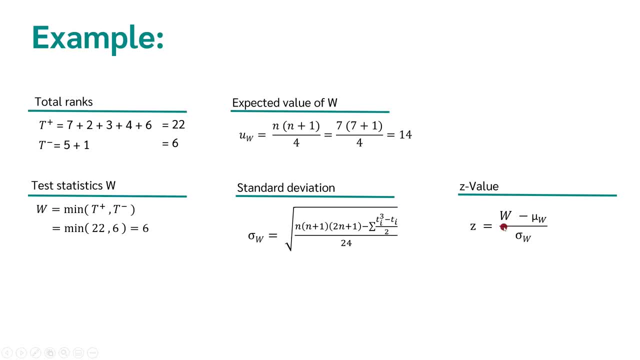 W minus µ and dividing that by the standard deviation. So we compare the value that would be expected if there was no difference with the value that actually occurred. Note that if there are more than 25 cases, normal distribution is assumed, in which case we can calculate. 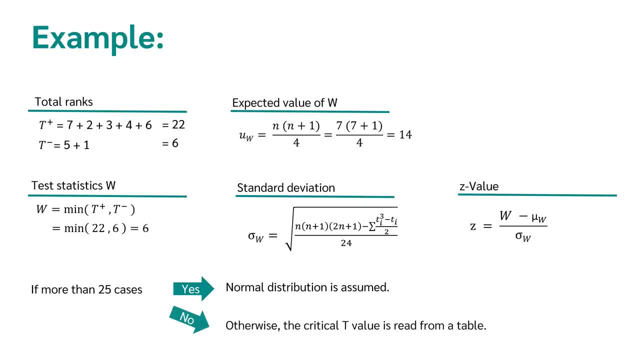 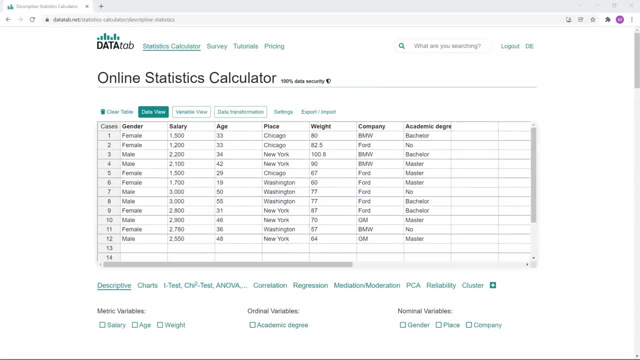 the Z-value. using this formula, If there are less than 25 values, the critical t-value is read from a table of critical t-values. Therefore, in our case, we would actually use the table. Now I will show you how you can easily calculate the Wilcoxon test online, And then I will 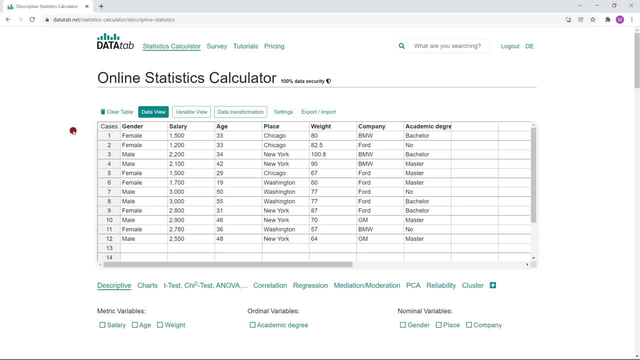 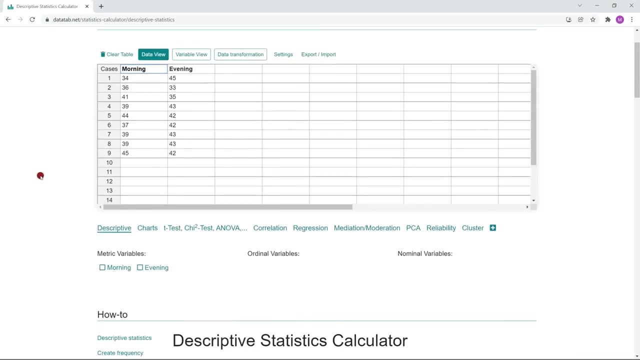 go into why you should always prefer the dependent t-test to the Wilcoxon test, if it's possible. In order to calculate the Wilcoxon test, simply go to datadepnet- you will also find the link in the video description- and you copy your own data into this table. Then you click. 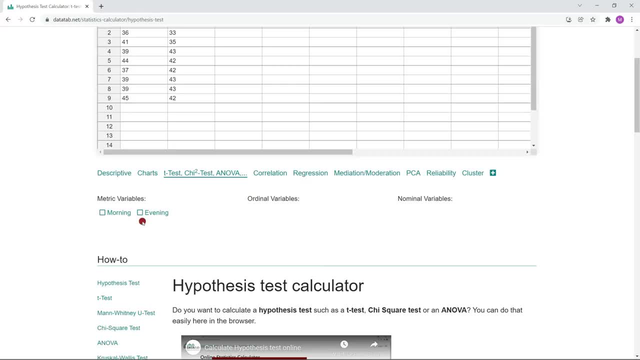 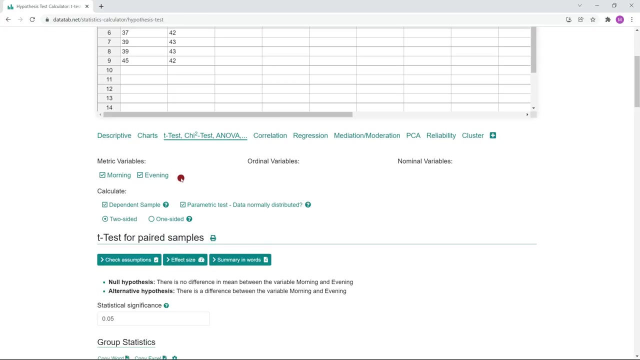 on this tab and you will see the names of all your variables. Underneath this tab, many hypothesis tests are summarized and Datadep automatically suggests the appropriate hypothesis test for your data. If you now select morning and evening, Datadep automatically recognizes that it is a dependent. 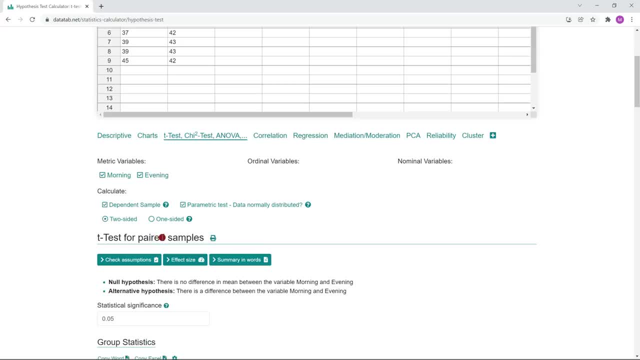 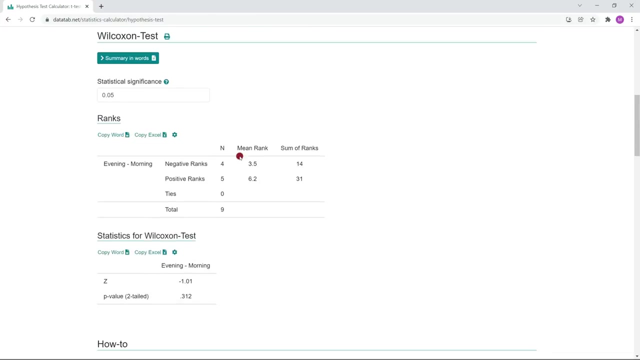 sample and calculates the dependent t-test. But we don't want to calculate a t-test, we want to calculate the Wilcoxon test. So we just click here. Now Datadep automatically calculates the Wilcoxon test. Here we can read the negative and positive ranks and here we see the z-value and the. 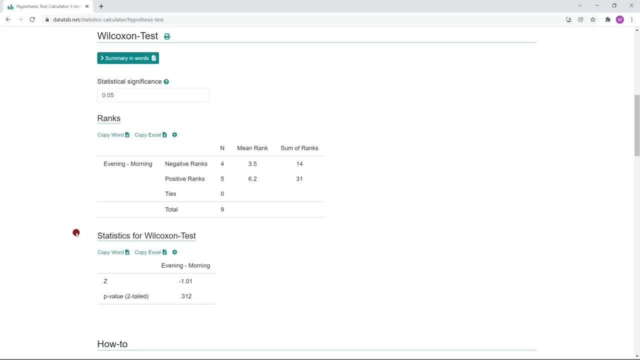 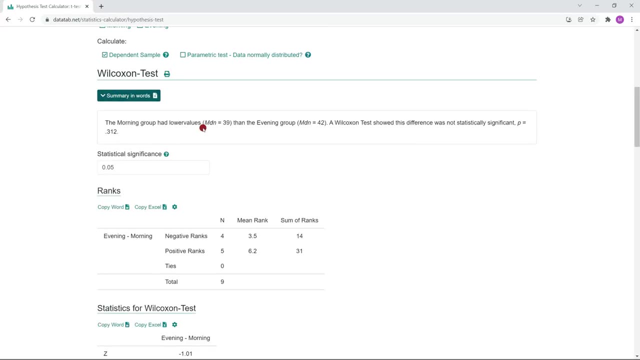 p-value. If you don't know exactly how this is interpreted, just look at the summary in words. It says that the morning group had lower values than the evening group And a Wilcoxon test showed that this difference was not statistically significant. p equals .312.. 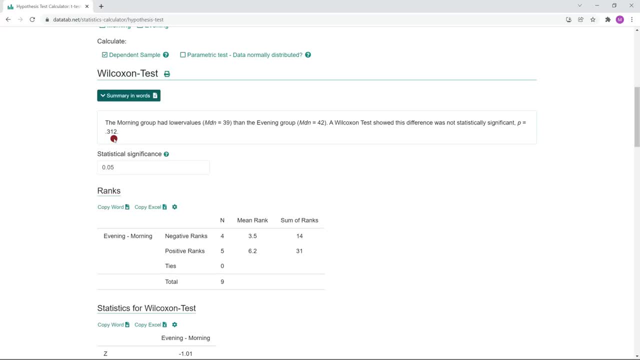 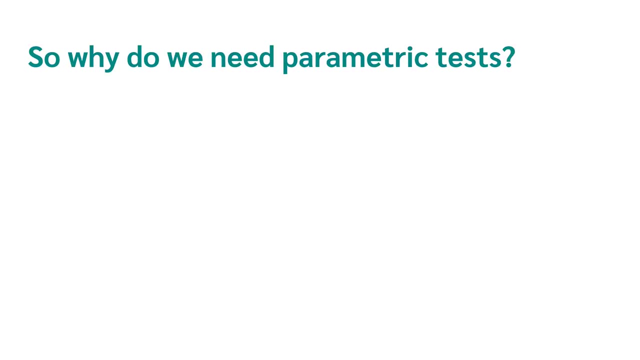 And now we come, as promised, to the point why you should always prefer a parametric test, for example the t-test, to a nonparametric test. We already discussed that the Wilcoxon test has fewer requirements than the t-test.